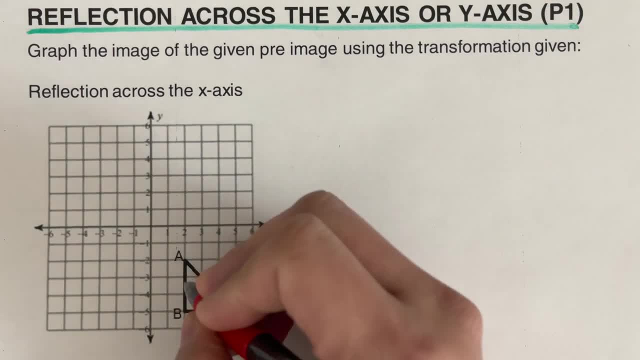 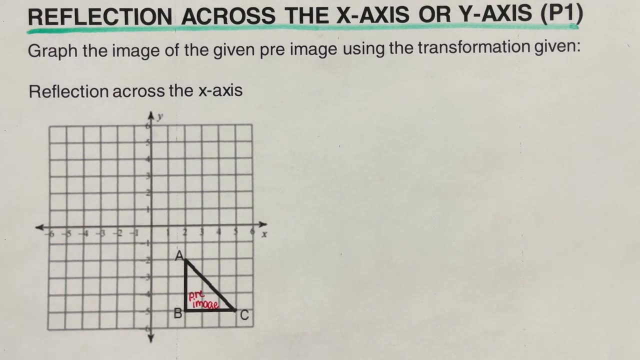 to come up with an image. So this one right here is called a pre-image, So I'm just going to label that down here. So that's the pre-image. Again, pre-image means it's the original figure. So then if we have the pre-image right here, we are supposed to reflect it across the x-axis. So if we have 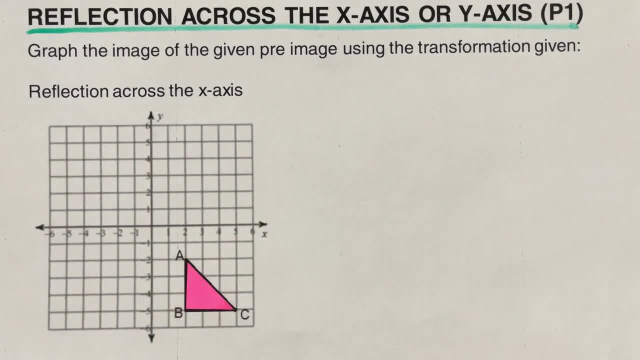 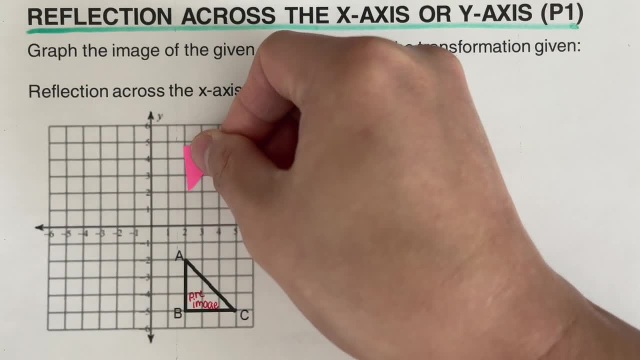 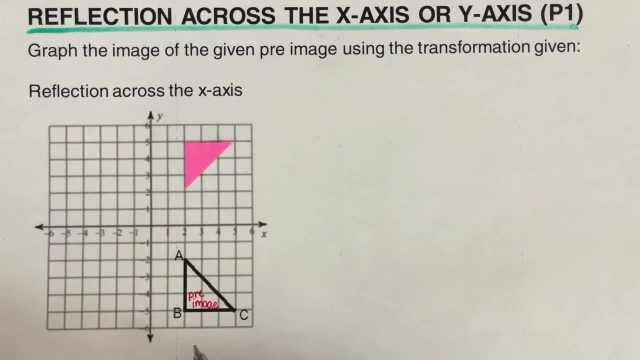 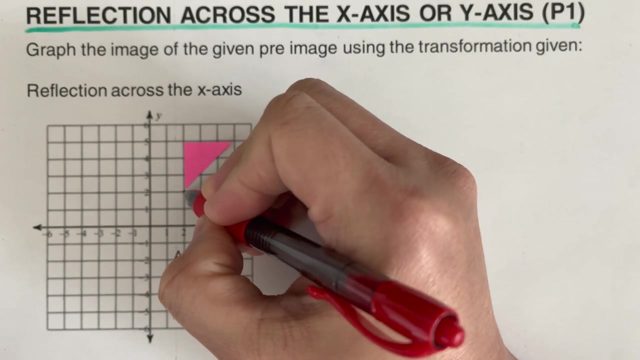 this original picture. We flip it across the x-axis. So if I were to flip this triangle, it's going to go up here. So this will be the location of our image after reflecting it across the x-axis or after we flipped it across the x-axis. So pretty much this will be our point A. Since this is our A, it was. 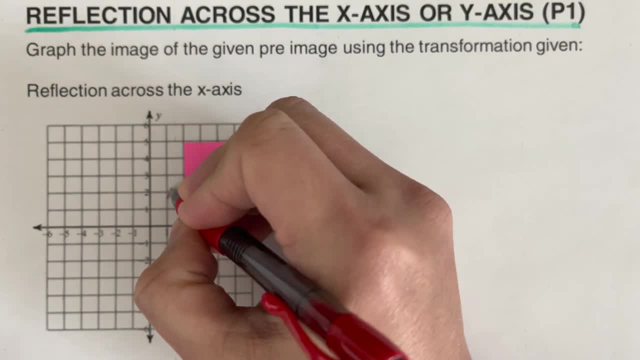 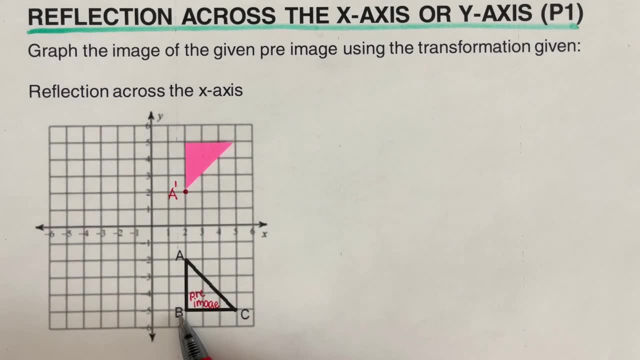 reflected across. It was flipped, So this will be our A. Again, prime represents the image or the new picture, And this is our B. If it doesn't have a prime, then that means that's the original coordinate, So that means we reflect it across. 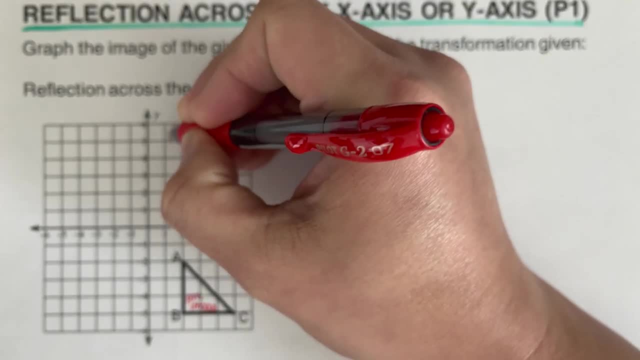 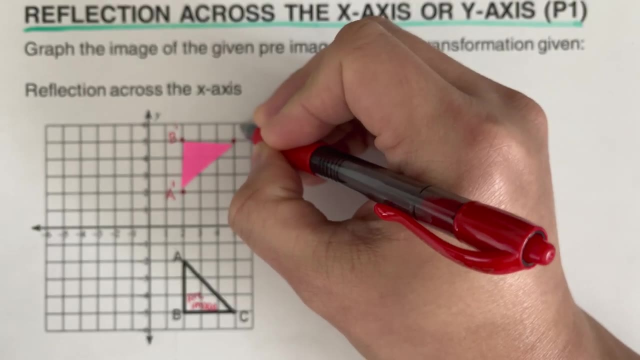 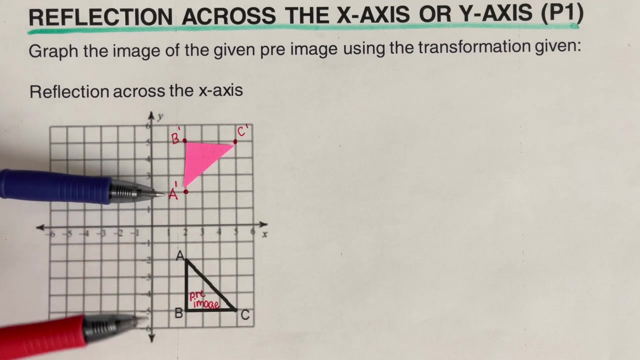 So this will be our B prime, And so this one right here would match up to C prime. So pretty much what's going on here is that it was flipped. So this is our A And this is our A prime, This is our B And this is our B prime, This is our C And this is our C prime. 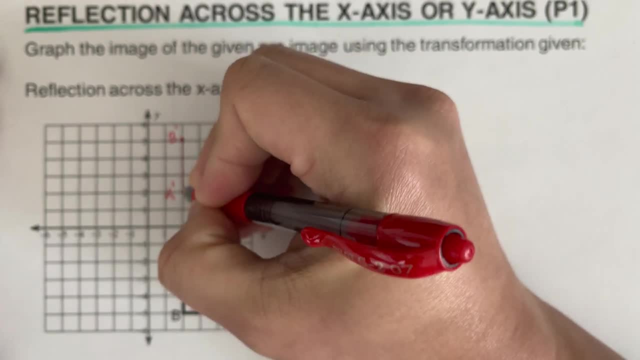 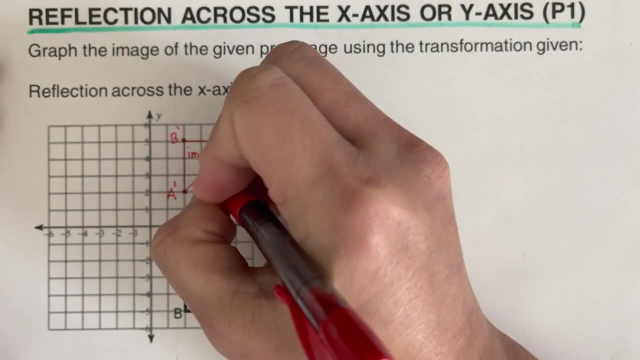 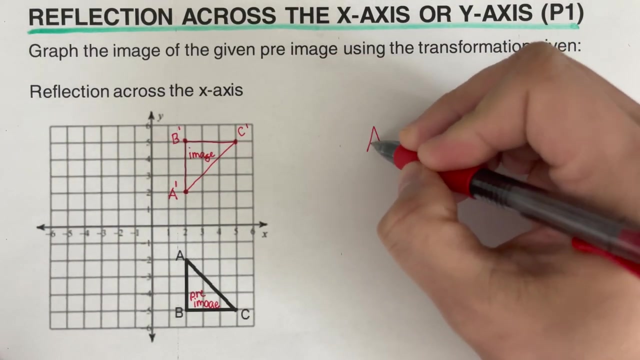 So then, if we are going to draw the triangle here, which is the reflected triangle, or we call this as our image, So this is our image, right here- So then we go ahead and say that the coordinates for the image would be: We write A prime, B prime and C prime. Again, these are the coordinates. 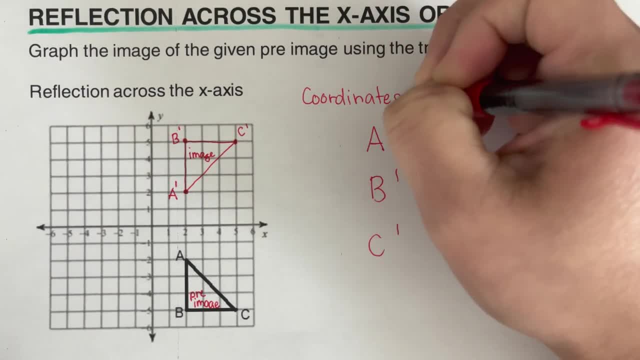 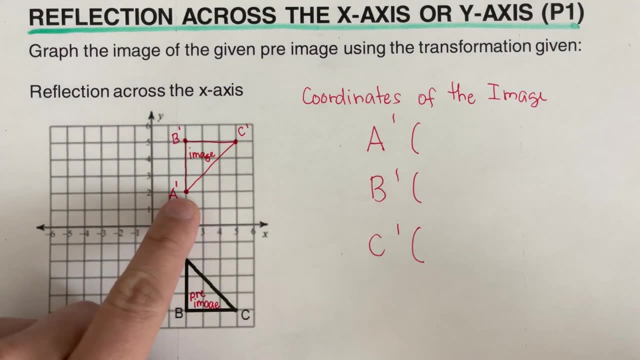 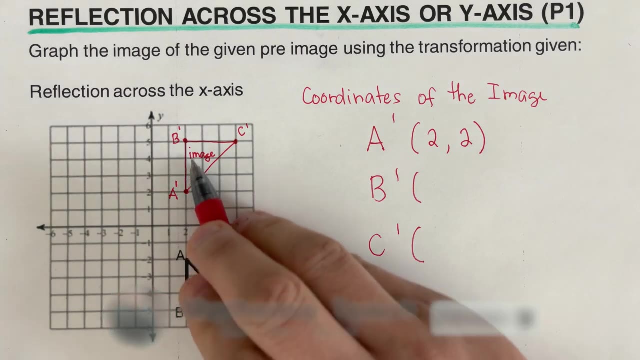 Of the image. Okay, So looking at this picture right here, our A prime is at 2, 2.. So I'm gonna write 2, 2 right here, And our B prime is located on 2, 5.. So that's 2, 5.. And our C prime is located on 5, 5.. 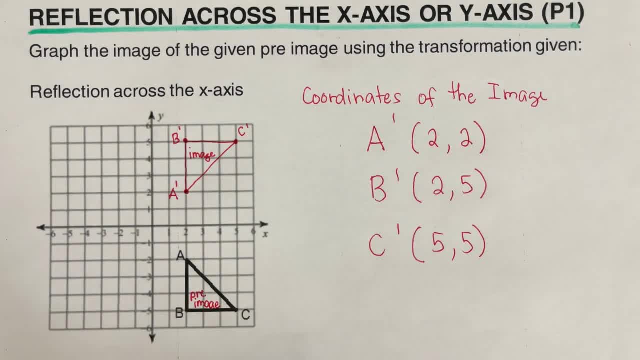 So this is 5, 5 right here. Notice that the distance from the x-axis to each of the vertices here are equal. What does that mean? So the distance from the x-axis to A is 2 units here, And that's also 2 units to A prime. 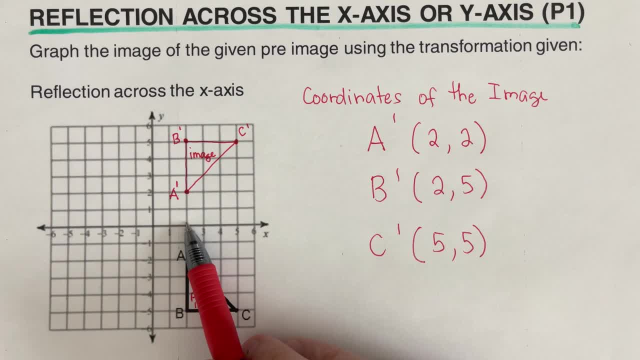 The distance from B prime to the x-axis would be 1,, 2,, 3,, 4, 5.. That would also be 5 for the B here. So that's the x-axis: 1,, 2,, 3,, 4, 5.. So pretty much when we say reflection. 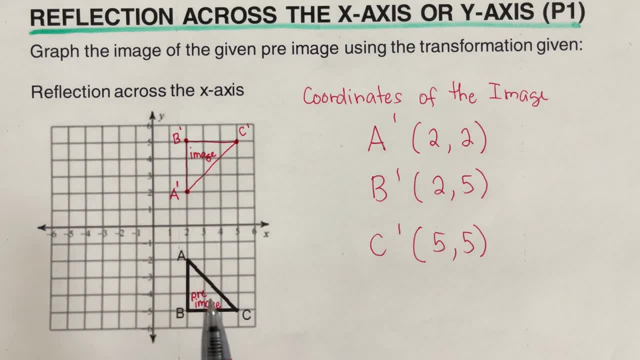 The distance of the image and the distance of the pre-image would be the same from the x-axis or from the line of reflection. At this time, I would encourage you to pause this video and try this problem out on your own And, when you're done, Pause it and check your answer. 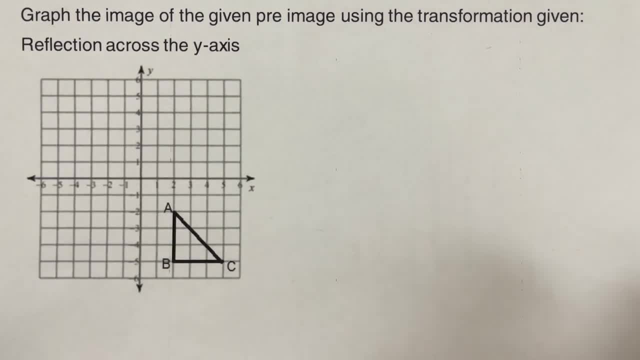 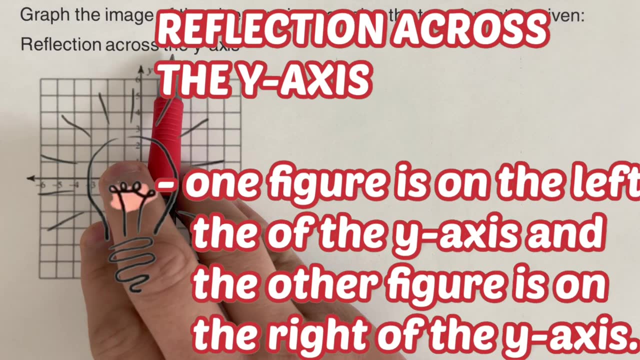 Okay, So we go over the problem here. So we're supposed to reflect this across the y-axis. Now, please remember that when we say reflection, Please remember that when we say reflection, Please remember that when we say across the x-axis, one figure is on the left of the y-axis and the other figure 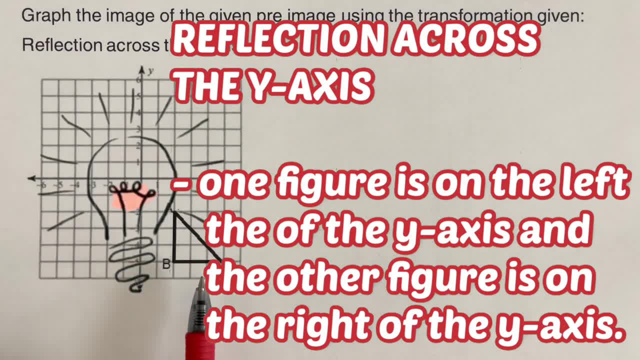 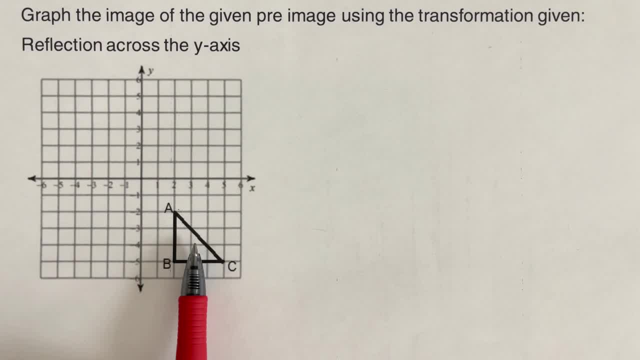 is on the right of the y-axis. so pretty much right. here we have a figure on the right of the y-axis. it says y-axis. we're supposed to draw another figure that is on the left of the y-axis. so, without having to use a picture, we can actually 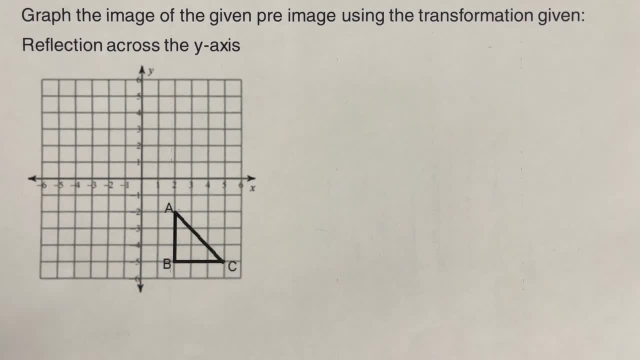 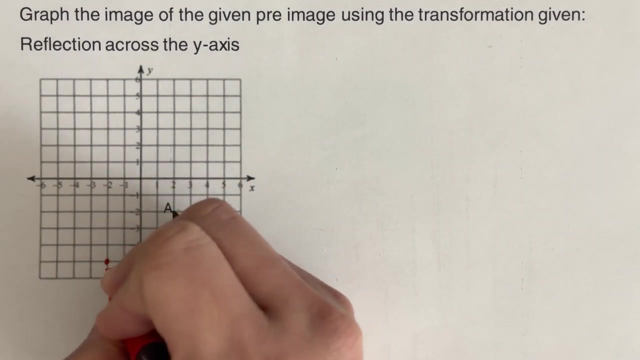 draw, or we can actually plot the vertices of the triangle on the other side by counting the distance from the y-axis. so pretty much, if this is our y-axis right here, we go ahead and say that is one to two units to the right. so I go two units to the left, one two. so this will be our B Prime, and so we do. 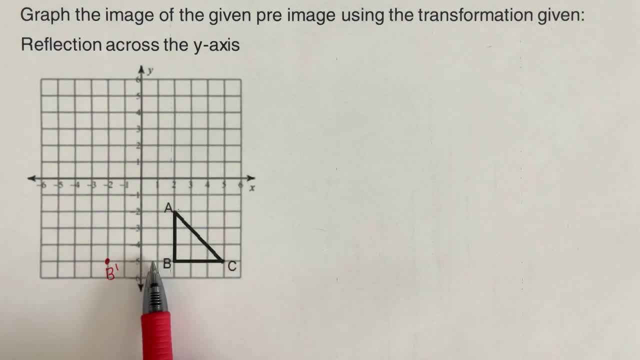 the same thing for C. if we count C from the y-axis, that would be one, two, three, four, five, five units to the right. so I go five units to the left to get C from. so that's gonna be one, two, three, four, five. so this is where our C Prime.